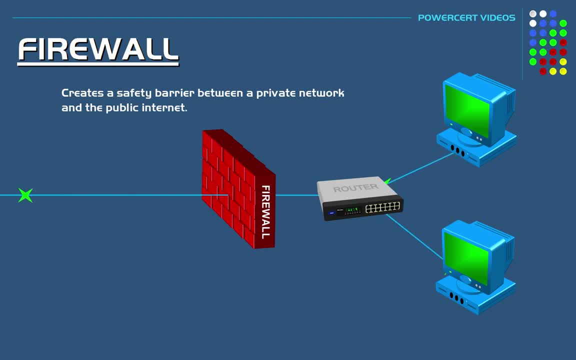 create a safety barrier between a private network and the public internet, Because out on the internet there's always going to be hackers and malicious traffic that may try to penetrate into a private network to cause harm, And a firewall is the main component on the network. 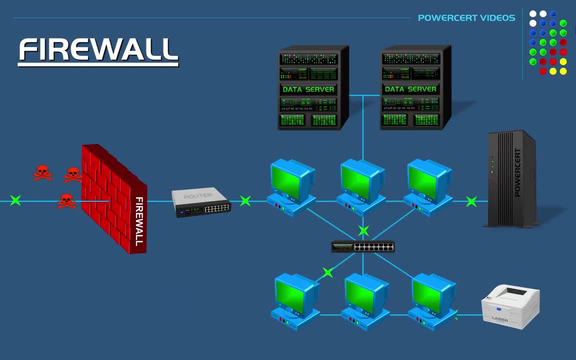 to prevent this. And a firewall is especially important to a large organization that has a lot of computers and servers in them, Because you don't want all those devices accessible to everyone on the internet where a hacker can come in and totally disrupt that organization. So that's. 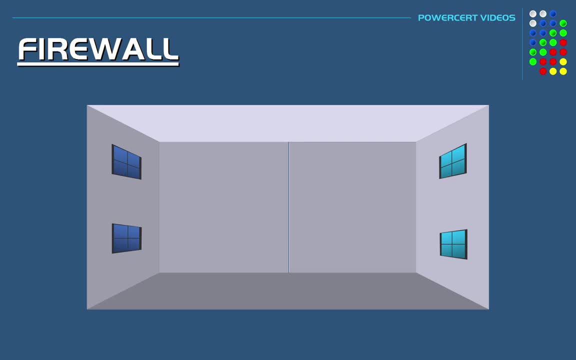 why you need a firewall- a firewall to protect them. So a firewall that's used in computer networks is very similar to how a firewall works in a building structure. In fact, that is where the word firewall came from. A firewall in a building structure provides a barrier so that in the event of an actual fire, 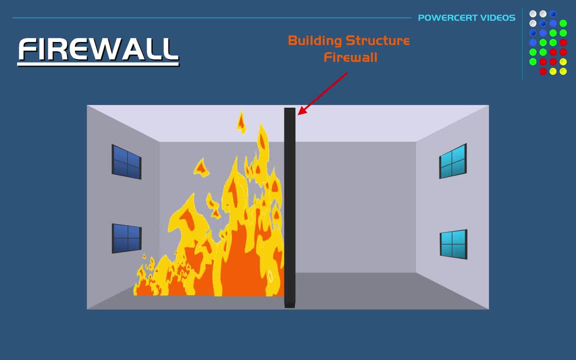 on either side of the building. the firewall is there to keep the fire contained and to keep it from spreading over to the other side. So the firewall is there to keep the fire from destroying the entire building. But if the firewall wasn't here, the fire would spread over to the other side. 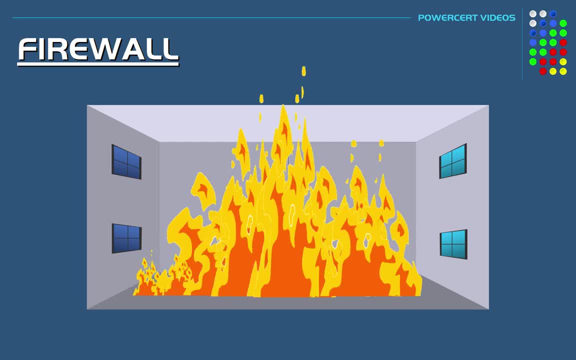 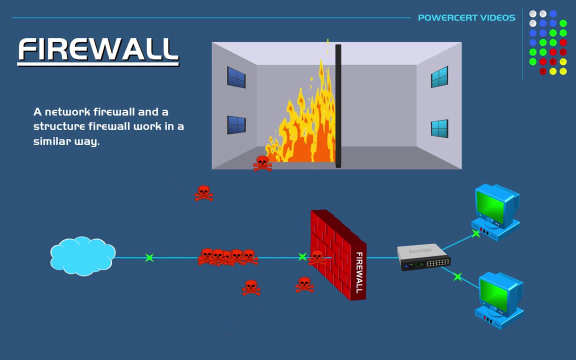 and then the whole building would be destroyed. And a network firewall works in a similar way as a structure firewall. It stops harmful activity before it can spread into the other side of the firewall and cause harm to a private network. So in today's high-tech world, a firewall is. 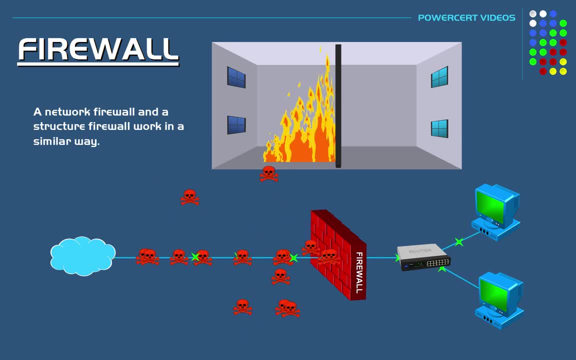 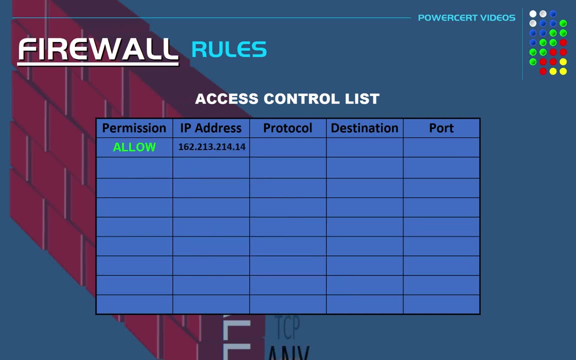 essential to every home, and especially in the business or an organization, to keep their network safe. Now, a firewall works by filtering the incoming network data and determines by its rules if it's allowed to enter a network, And these rules are also known as an access control. 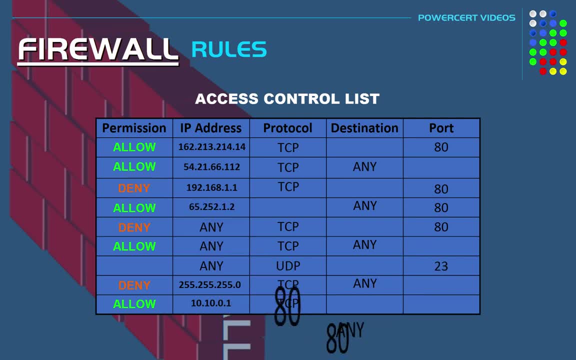 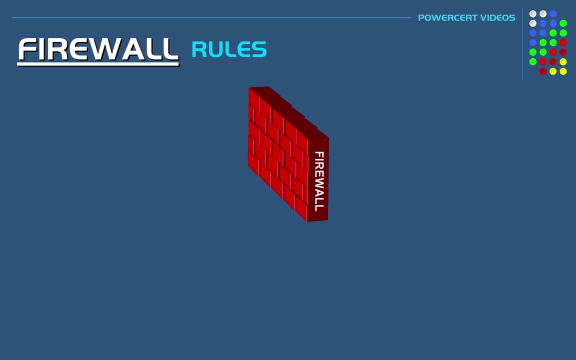 list. These rules are customizable and are determined by the network administrator. The administrator decides not only what can enter a network, but also what can leave a network. So these rules either allows or denies permission. So as an example, here we have a firewall that is. 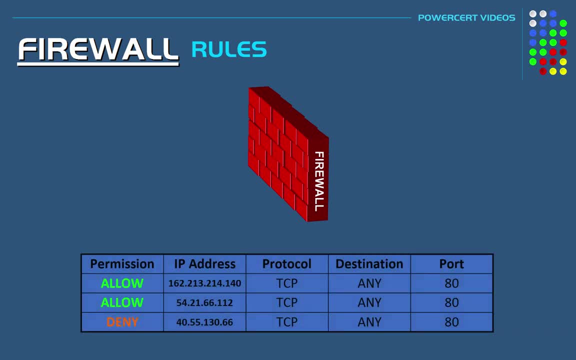 a firewall that is controlled by a network. So let's say we have some rules in a firewalls access control list and it shows a list of IP addresses that have been allowed or denied by this firewall And, as you can see, traffic from some IP addresses are allowed to enter this network but traffic from 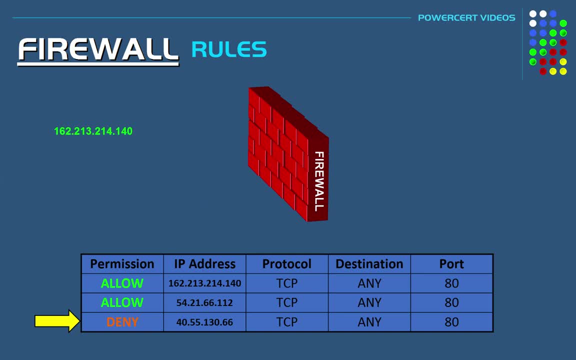 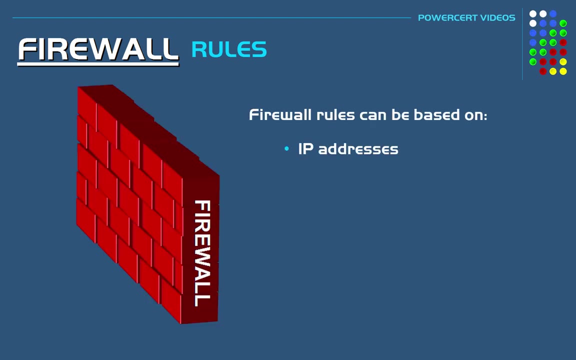 one IP address has been denied. So if traffic from this IP address try to get into this network, the firewall will deny it because of the rules that are set in the firewall. But the other IP addresses, the rules allow them. Now, firewalls don't just make rules based on IP addresses, but they can. 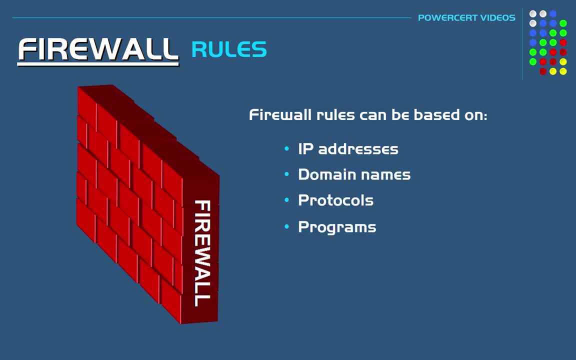 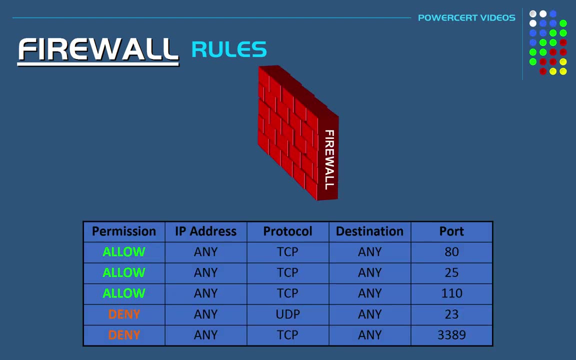 also make rules based on domain names, protocols, programs, ports and keywords. So let's say, in this example, the firewall rules are controlling access by port numbers And let's say that the rules have allowed incoming data, that's, using port number 80,, 25, and 110 and the data using those ports. 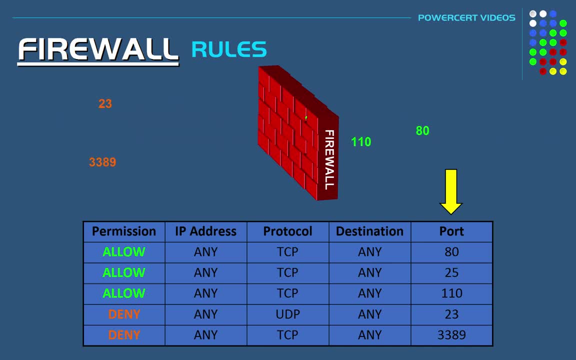 have been given access to this network. So let's say that the rules have allowed incoming data that's using port number 80,, 25, and 110 and the data using those ports have been given access to this network. So any incoming data that's using those ports can pass through the firewall. But also in this, 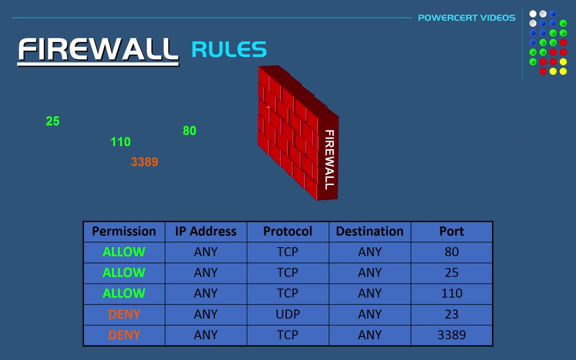 firewall. the rules have denied any data that's using port numbers 23 and 3389.. So any incoming data that's using those port numbers the firewall will deny access and it won't get past the firewall. So in a nutshell, this is how firewalls basically work. Now firewalls do come in different. 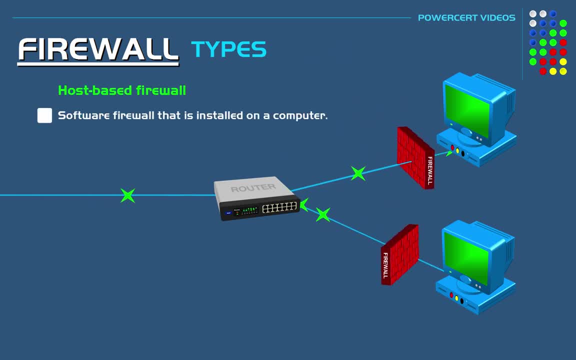 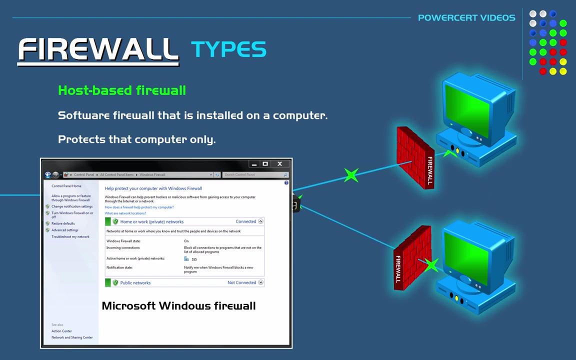 types, and one type is called a host-based firewall, And this is a software firewall. This is the kind of firewall that is installed on a computer and it protects that computer only and nothing else. So, for example, later versions of Microsoft operating systems come pre-packaged with a host-based firewall, And you can see that example here. And 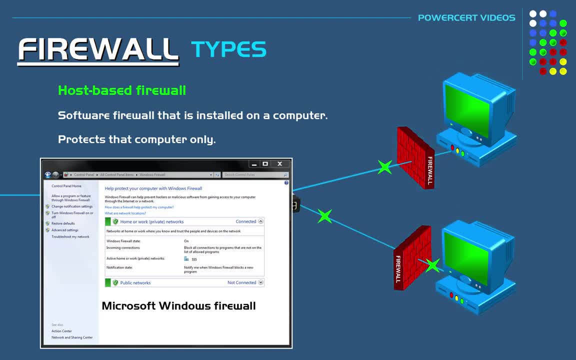 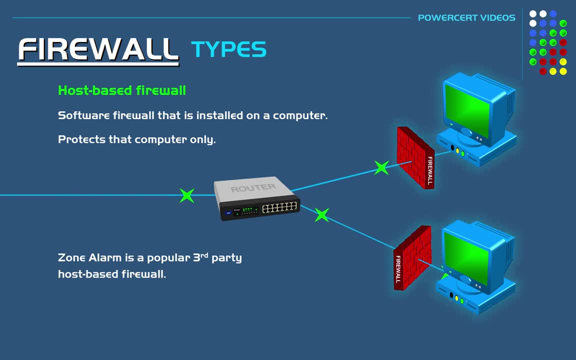 there are also third-party host-based firewalls that can be purchased and installed on a computer. So, for example, zone alarm, which is a popular third-party host-based firewall, And also a lot of antivirus programs will have a built-in host-based firewall And another type of firewall. 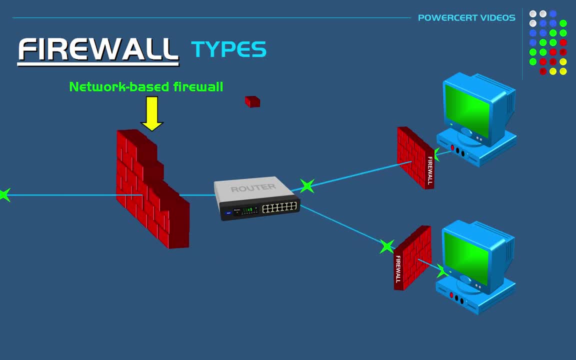 is called a network-based firewall. A network-based firewall is a combination of hardware and software and it operates at the network layer And it is placed between a private network and the public internet. But unlike a host-based firewall where it only protects that computer, a network-based